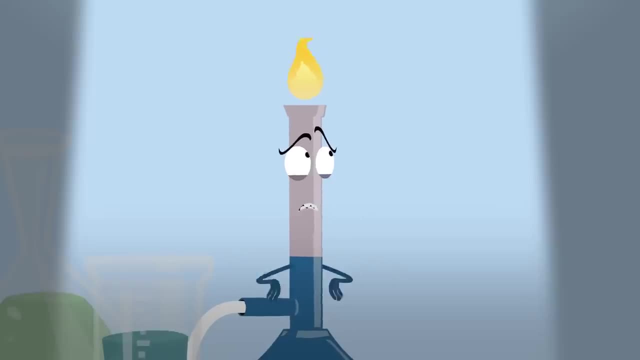 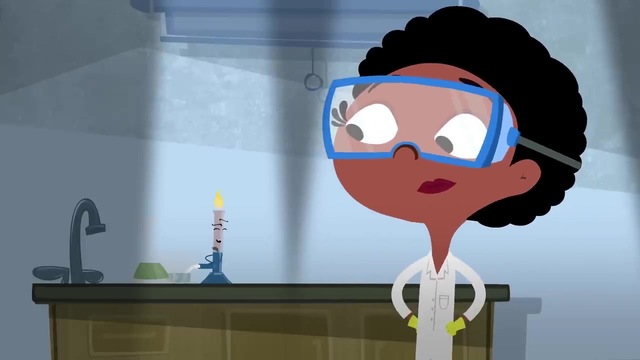 But you might be surprised how challenging this can be for students. Well, I'm trying to keep things simple by not getting into the nitty-gritty just yet, But that nitty-gritty is where it's at. Students tend to have a better understanding of chemical reactions. 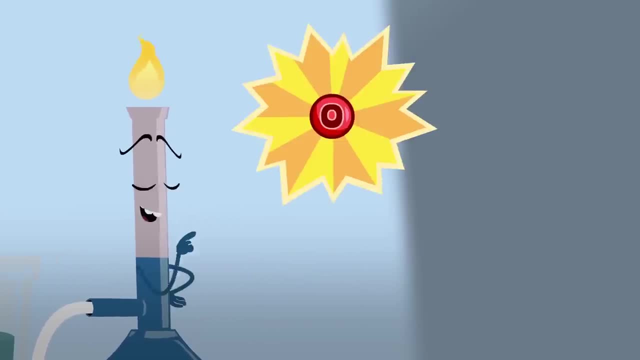 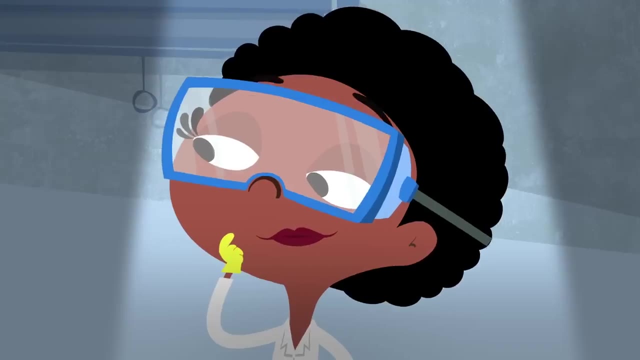 when they're asked to explain what they see in terms of atoms and molecules. This can begin with teaching the concept of a substance. So, instead of just saying that metal is producing rust, you might explain what makes up that metal. One of those things is called iron, made up of iron atoms. 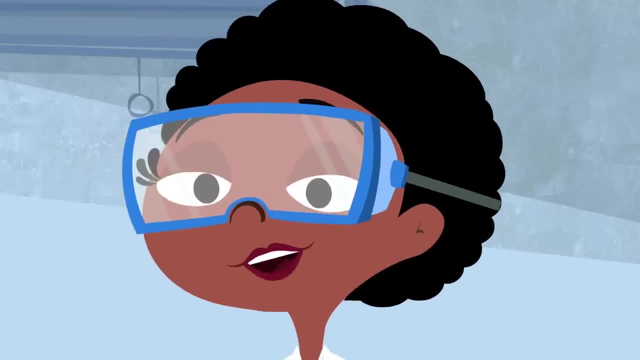 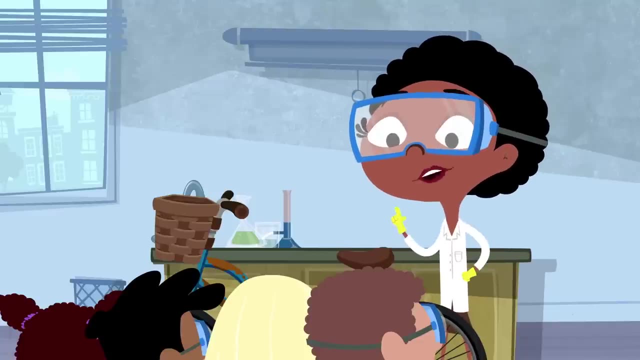 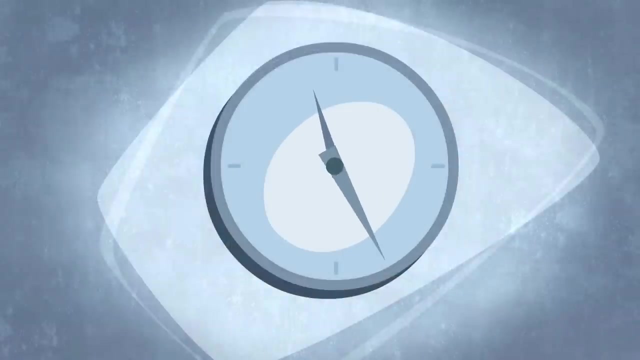 Give it a whirl. Okay class, Let's see if we can like. my spinning instructor says: dig deep and put the pedal to the metal. Who can tell me the difference between an atom and a molecule? So, as I was saying, the metal making up this bicycle contains iron. 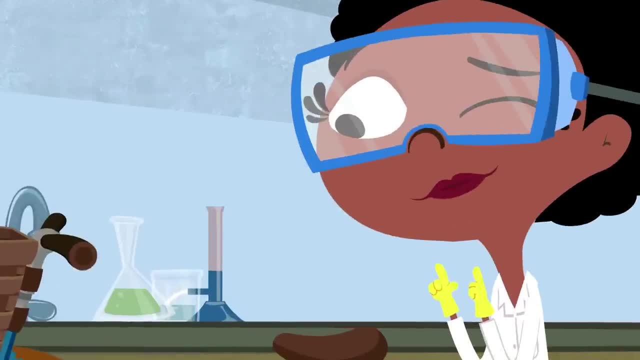 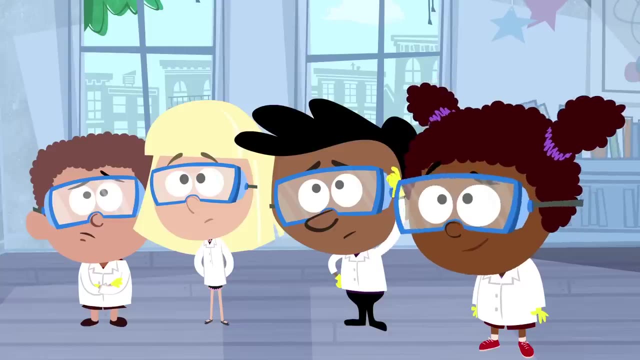 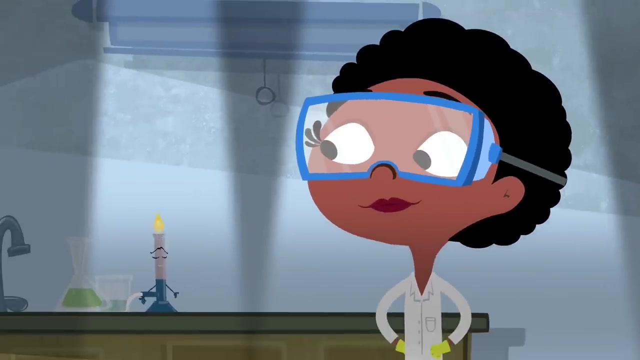 which is made up of iron atoms. Who are you winking at? These atoms can undergo a chemical reaction that produces rust. I think they're really starting to get it now. We're off to a grade A start, But we might be getting a little ahead of ourselves. 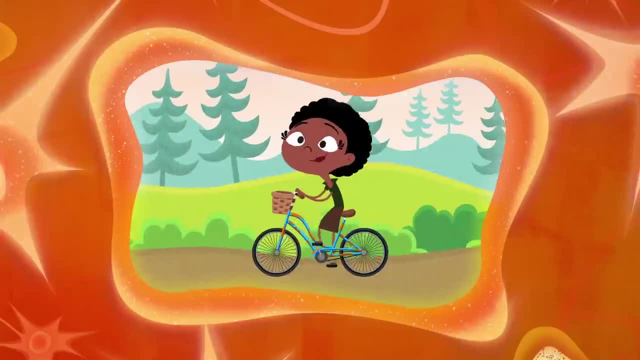 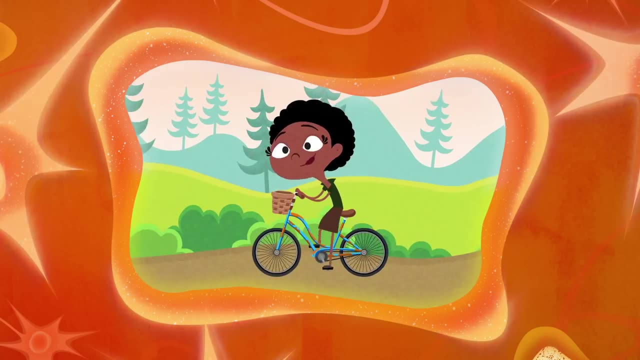 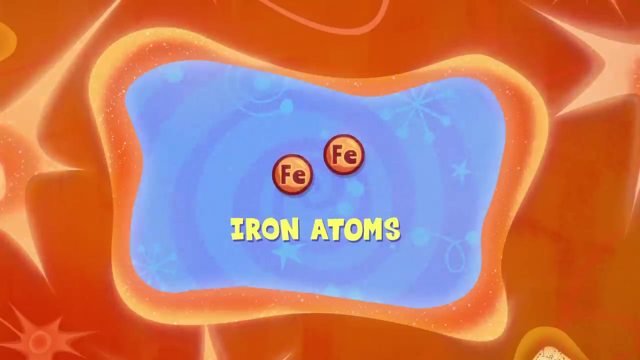 Let's take a peep inside Amar's noggin. hmm, These atoms can undergo a chemical reaction that produces rust. Okay, for the record, I'm much more graceful than that. See, Amar is just starting to understand what happens with atoms in chemical reactions. 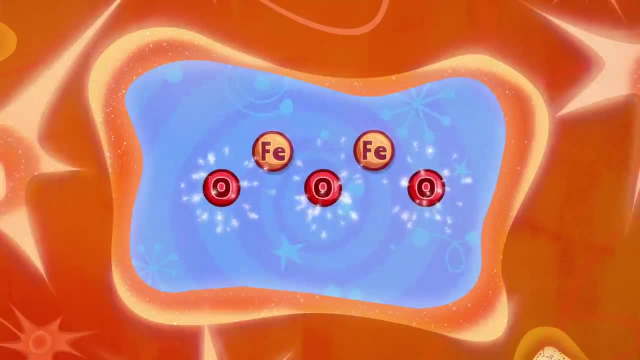 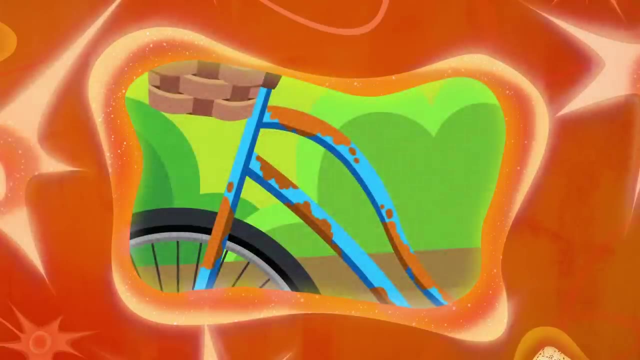 But, as you can see, it's not just about the metal, it's about the oxygen. Where'd those oxygen atoms come from? Well, he is right That rust is made up of more than just iron, But where did he think those atoms came from? 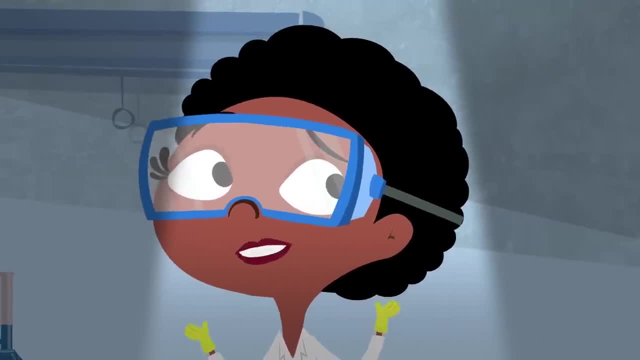 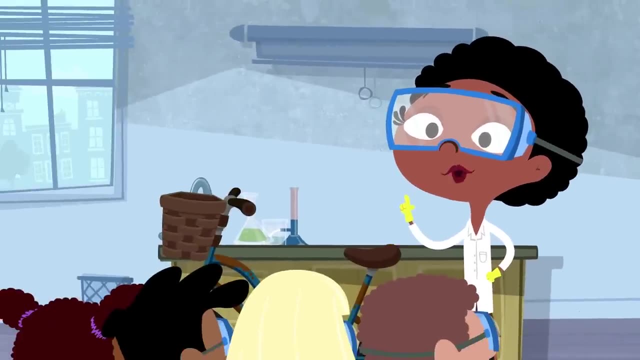 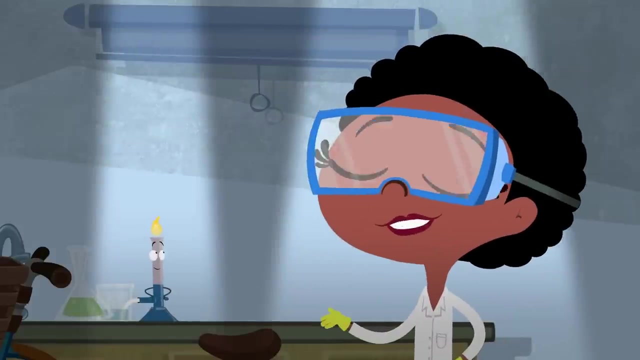 Hmm, I realize now that I wasn't very specific earlier. I should have said: the iron atoms in this bike combine with oxygen molecules from the air around us to produce rust. I think Amar is on a good path, But I've got a solution. 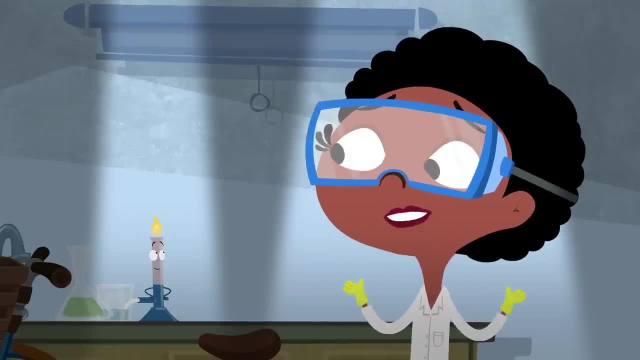 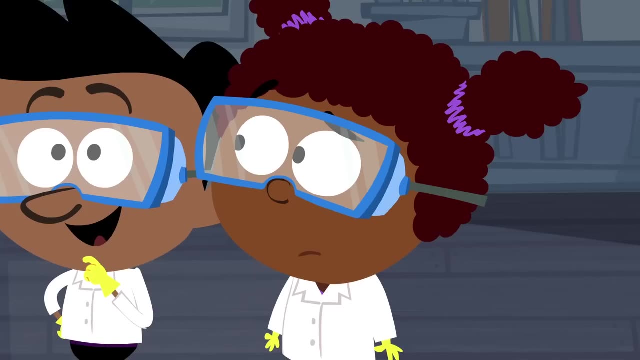 I've seen enough to know that doesn't mean all my students have landed in the same spot. Exactly the point I was just about to illuminate. Why don't we dive into Justine's perfectly shaped melon to see what she took from that? 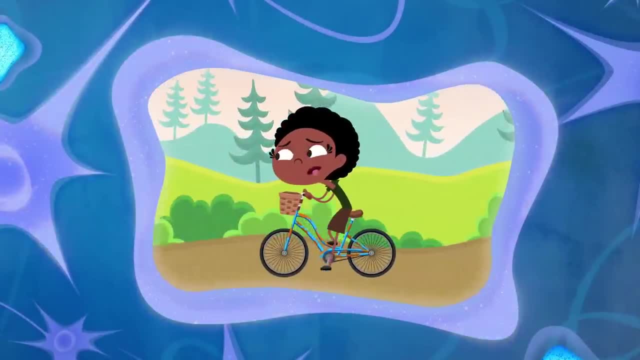 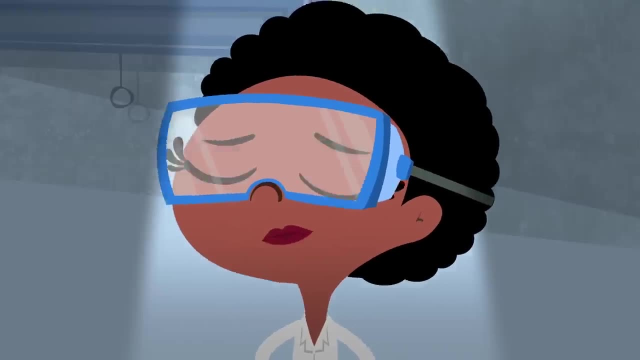 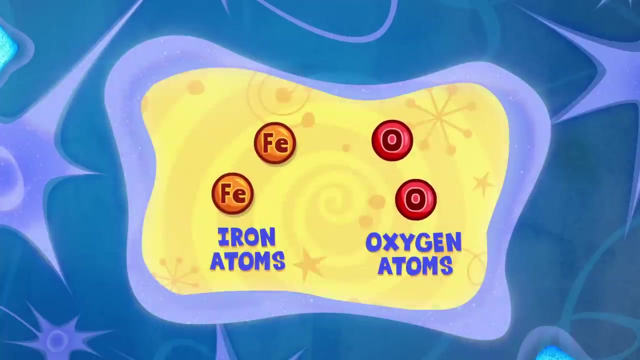 The iron atoms in this bike combine with oxygen molecules from the air around us to produce rust. Oh, come on. Just for the record, my nickname in spinning class is the Viper. See Justine's already thinking on the molecular level. 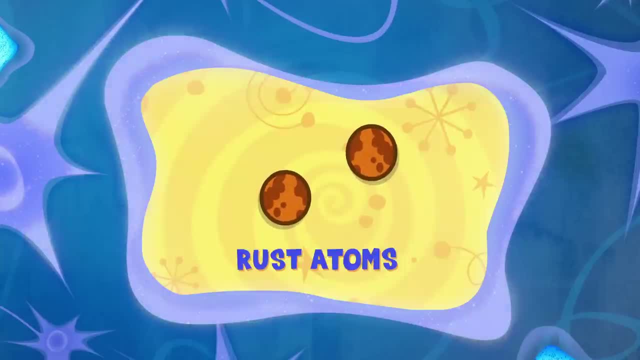 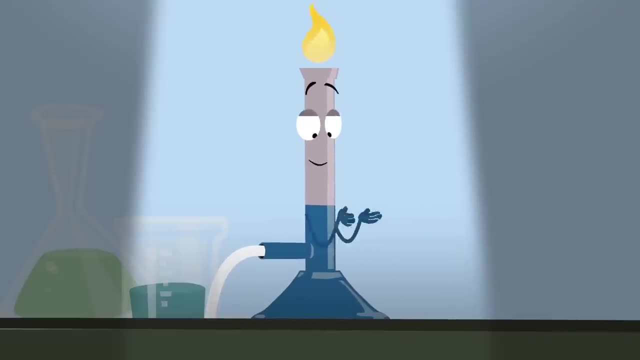 Rust atoms? That's not a thing. Neither are wallet-sized Hadron colliders, but that didn't stop me from pre-ordering one, just in case. Many students who hear about two substances combining imagine that they become something totally new, made out of different types of atoms. 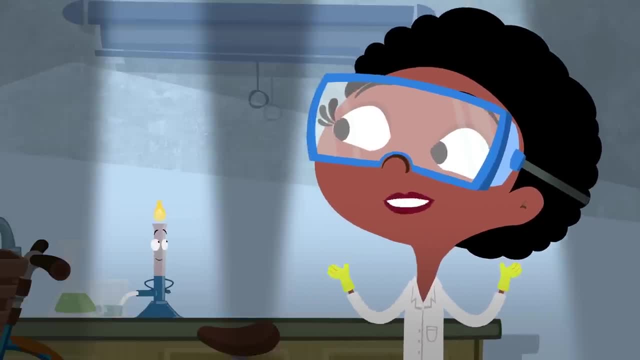 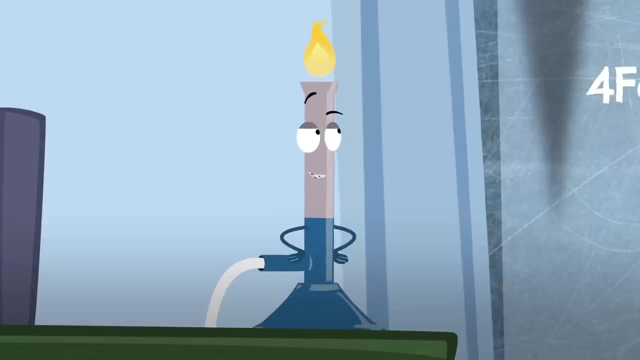 I noticed that Perhaps I can walk them through the chemical equation. Whoa there, There, Speedy McQuikerson. That's some of the fastest chalkboard riding I've ever seen. Was that chalk, dust or smoke? Not too bad eh. 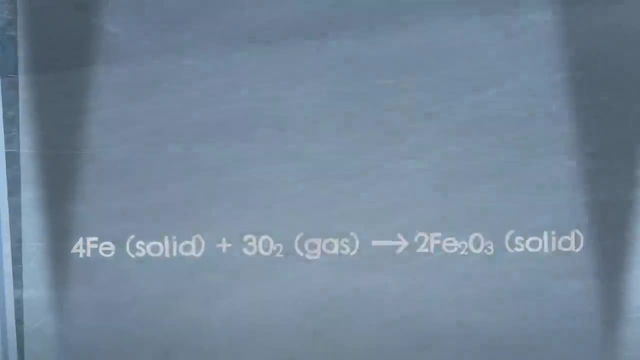 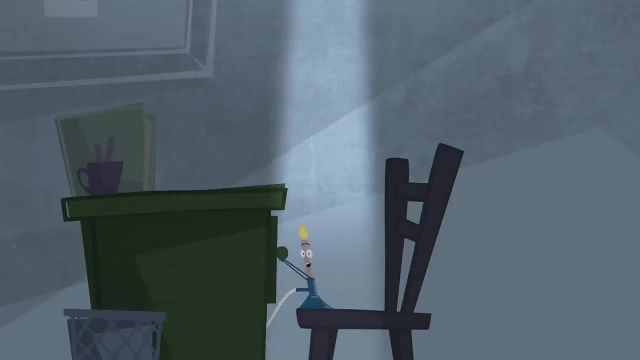 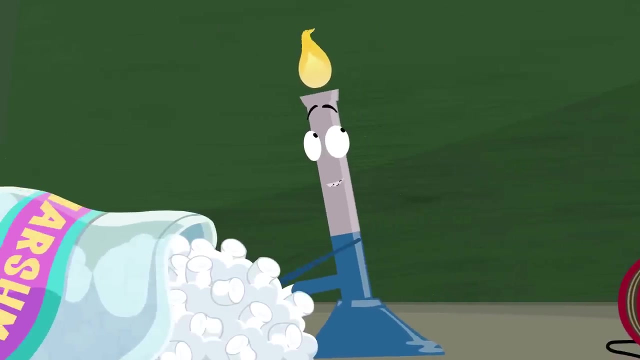 I feel like this will really help them understand what's happening. Not so fast there. the Viper- I mean talking about the chemical interactions from a molecular standpoint- is a good start, And seeing the interactions written out can help. but it's definitely an abstract concept and those symbols can be confusing on their own. 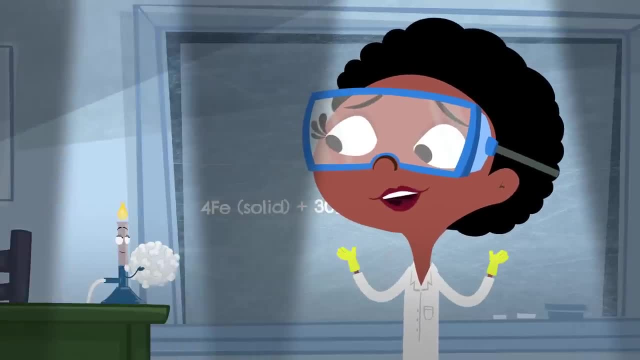 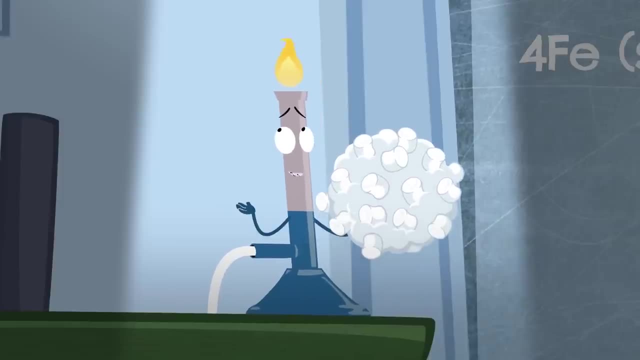 That's your solution. Marshmallows, When aren't they the answer? Seriously, though, having students use concrete visual models helps them to reason through how atoms rearrange into different molecules. You don't have any food coloring, do you? Uh, not on me. 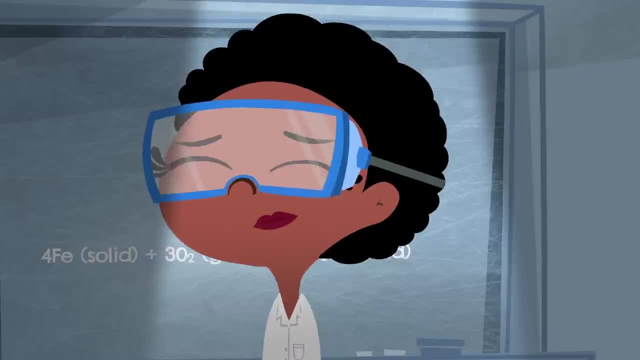 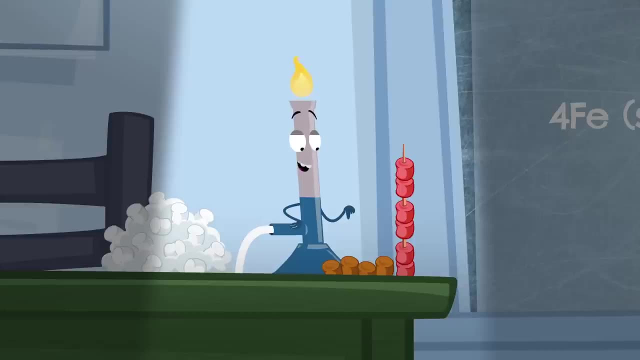 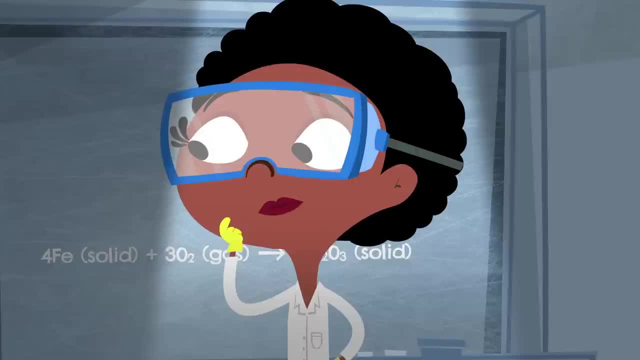 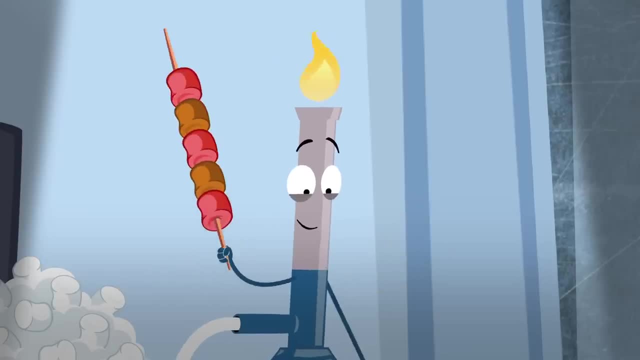 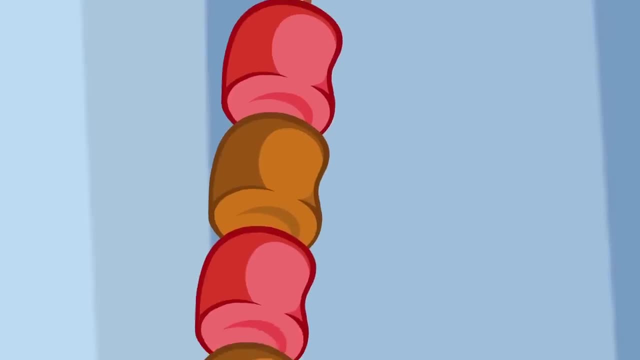 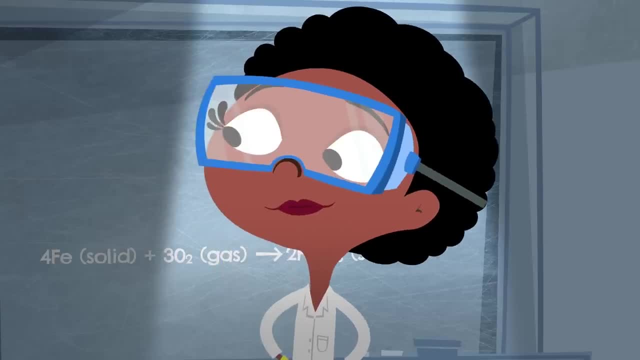 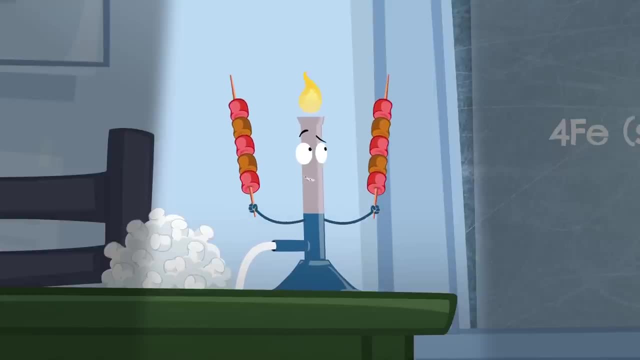 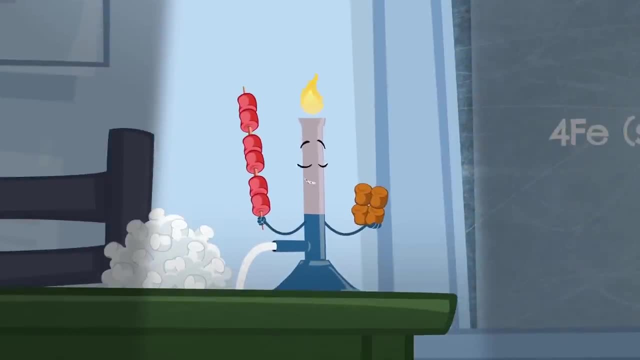 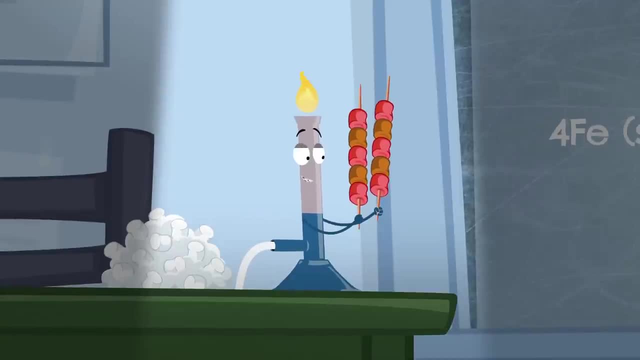 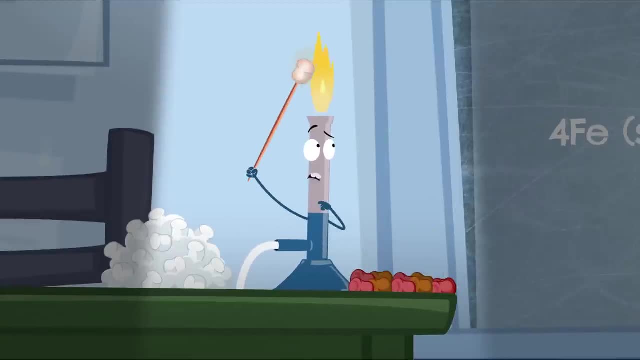 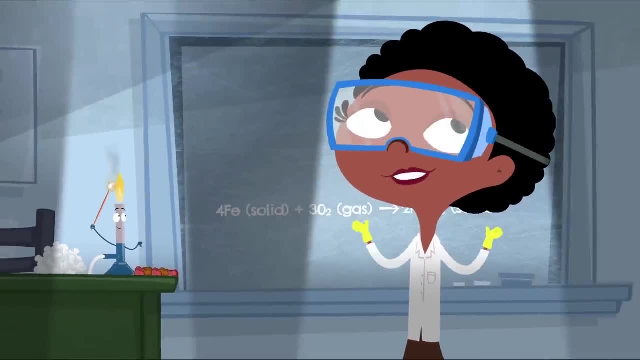 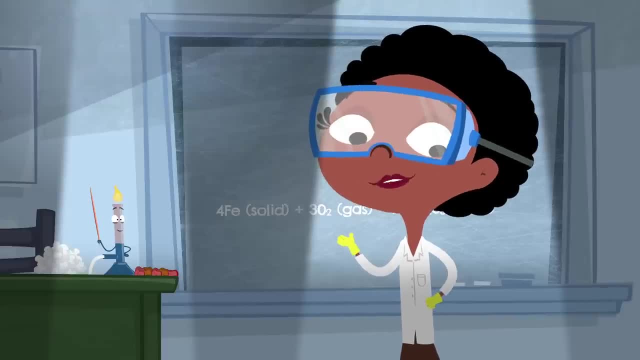 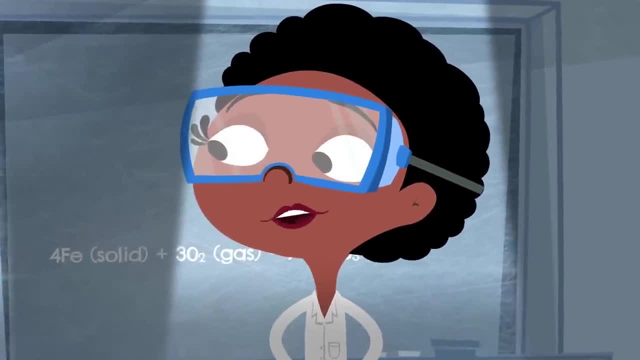 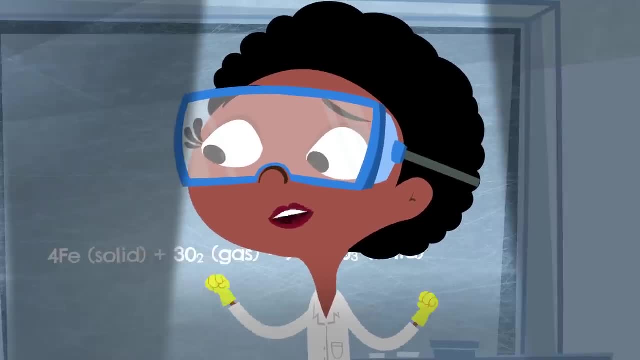 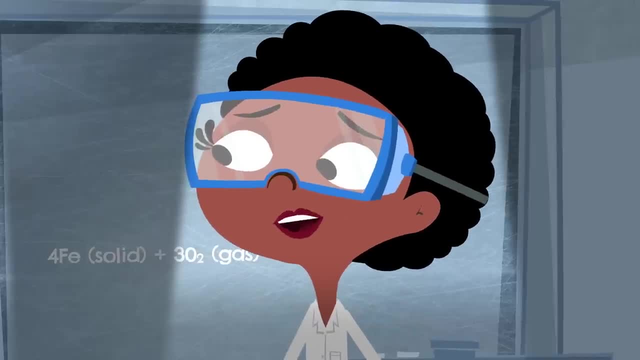 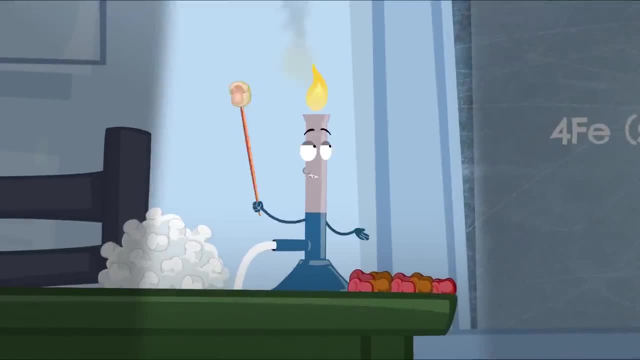 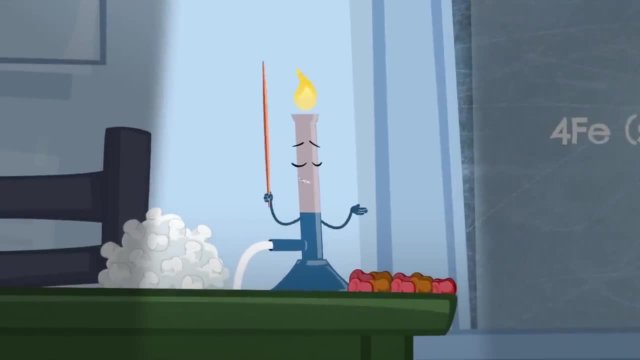 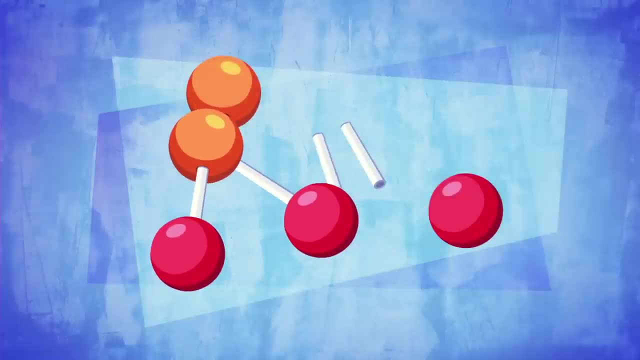 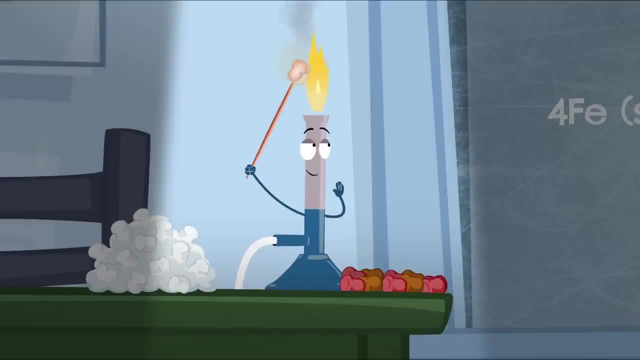 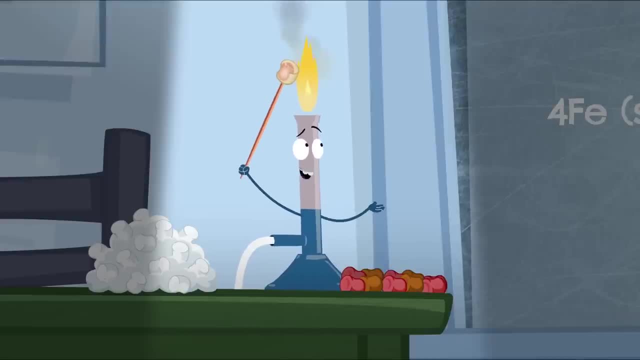 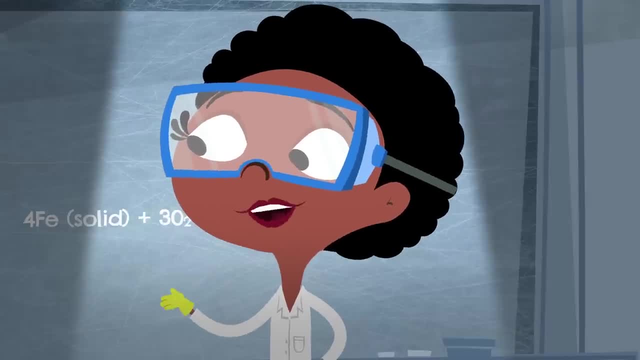 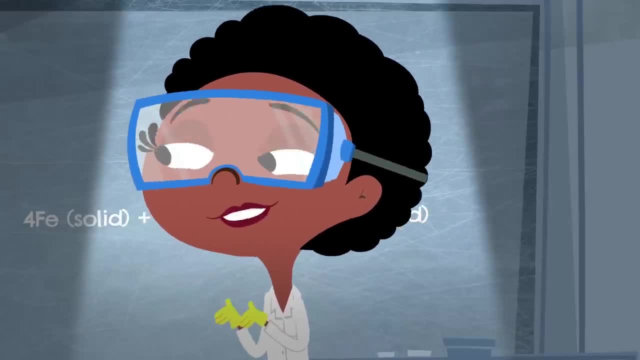 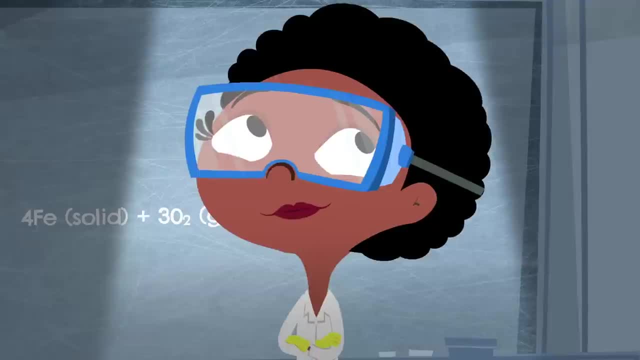 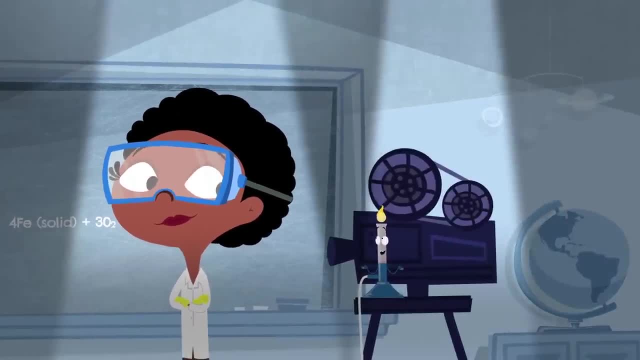 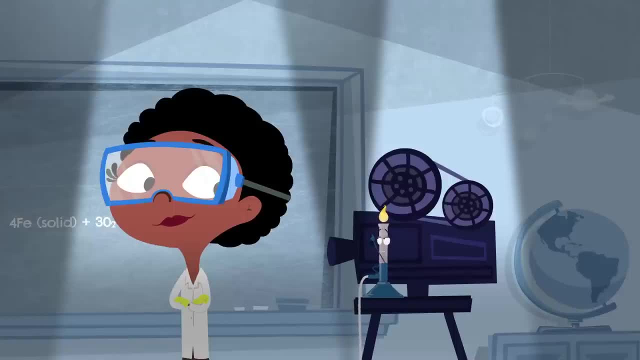 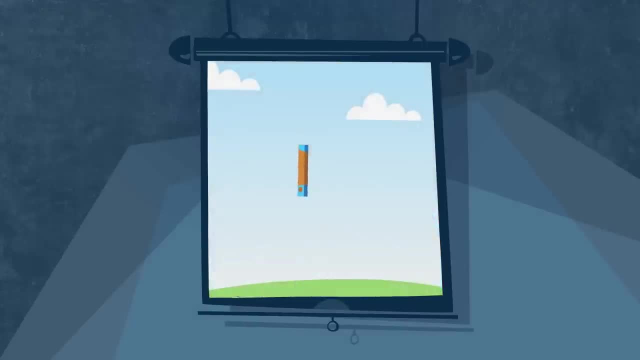 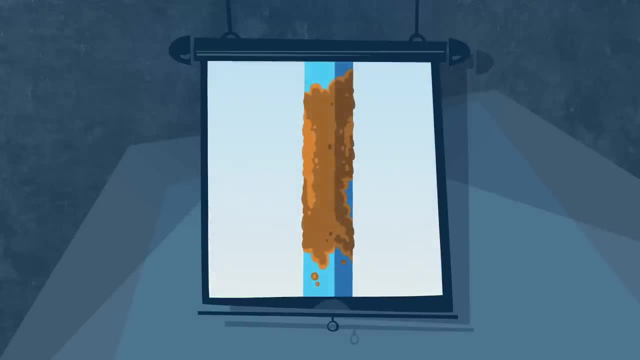 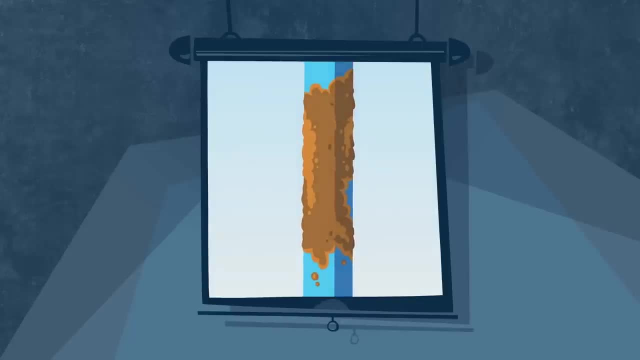 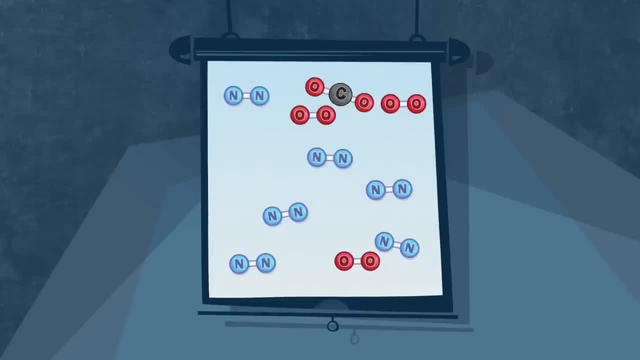 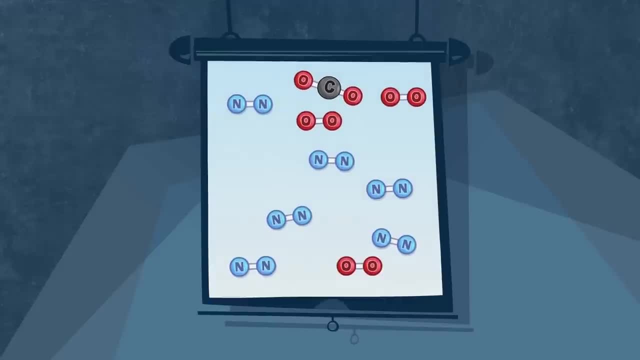 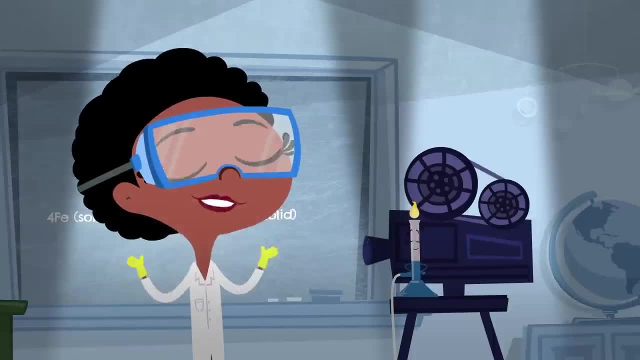 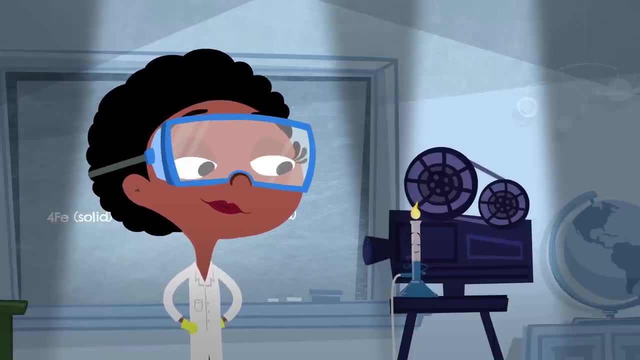 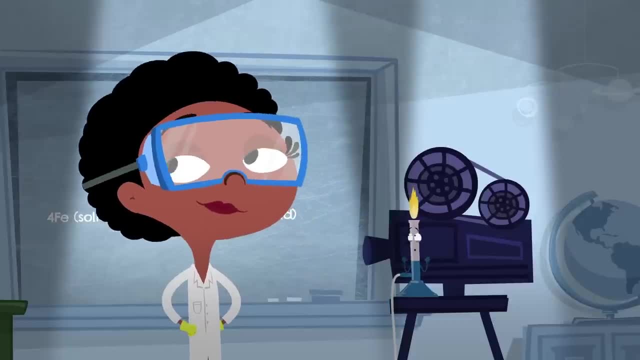 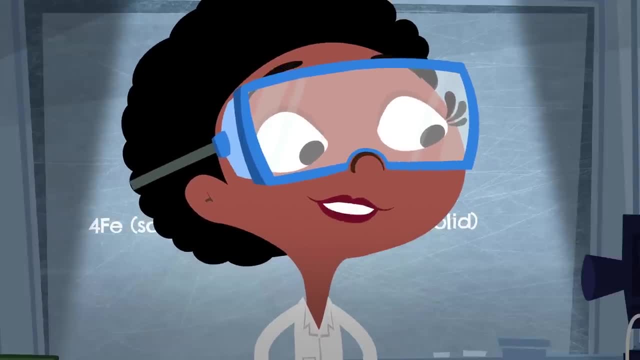 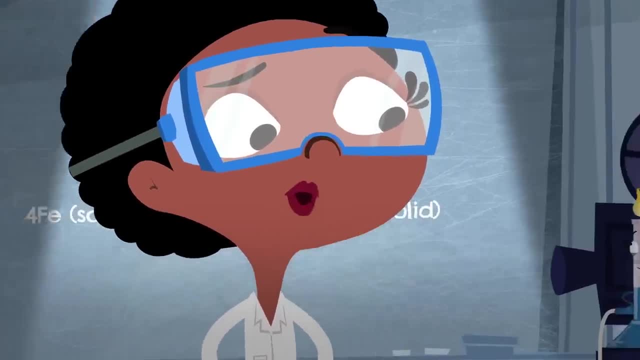 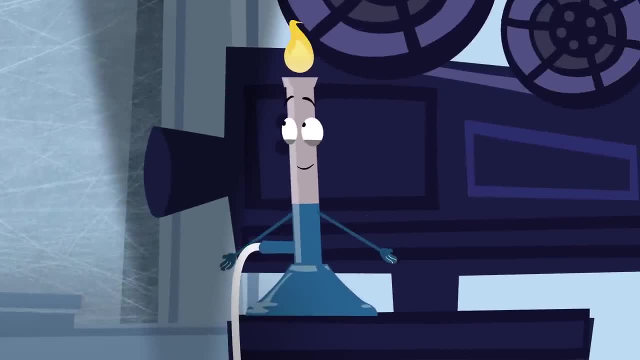 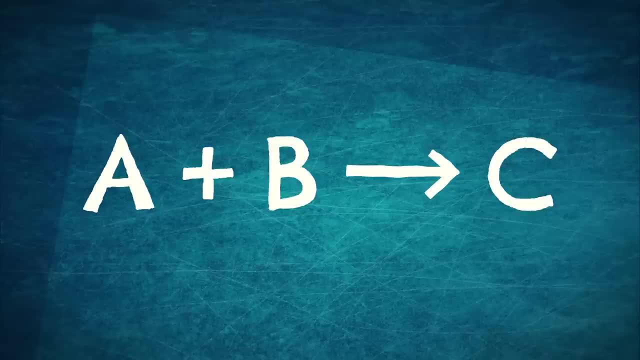 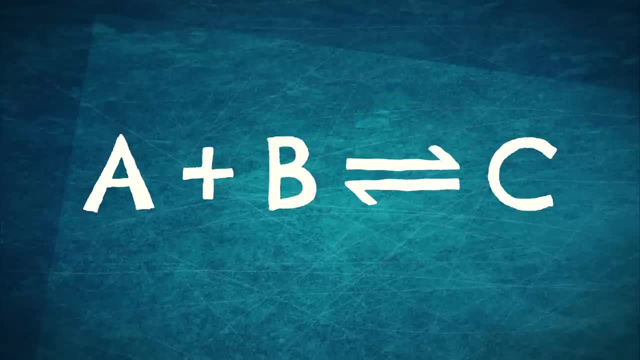 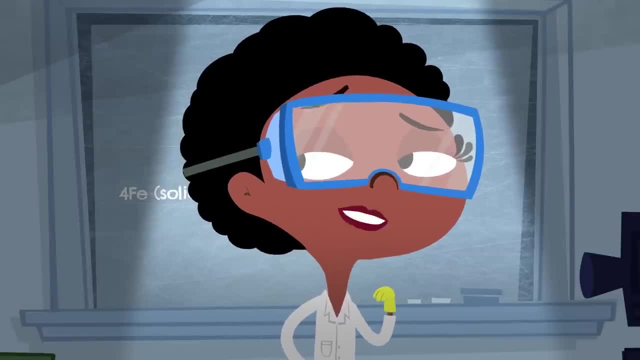 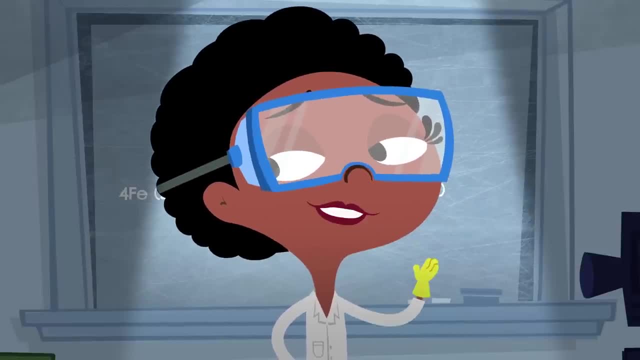 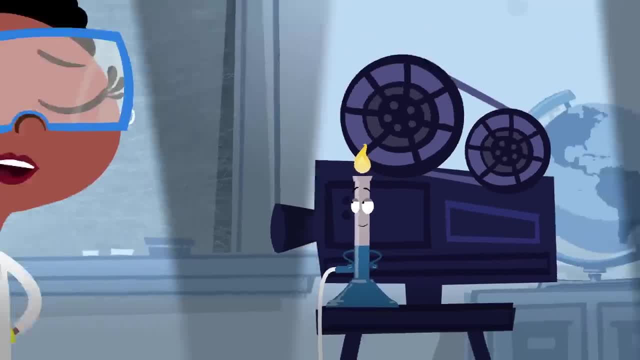 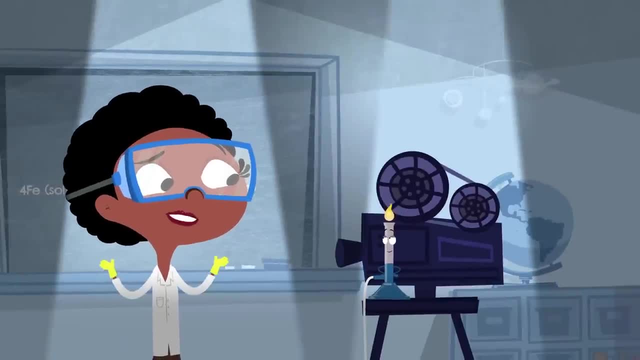 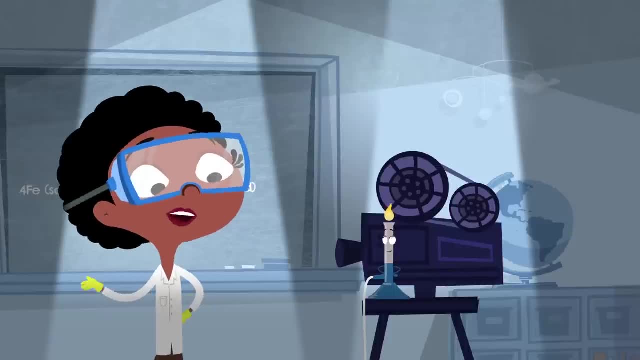 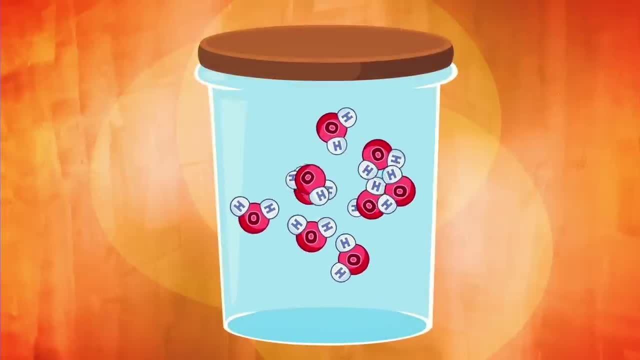 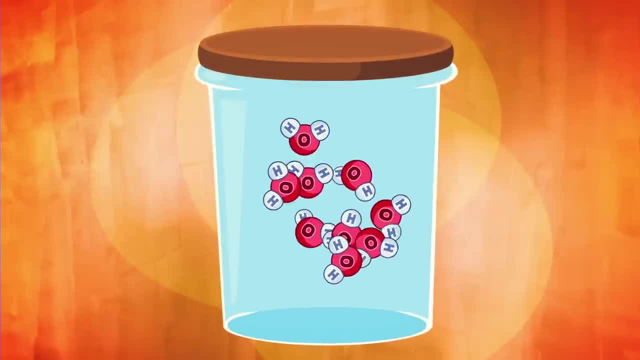 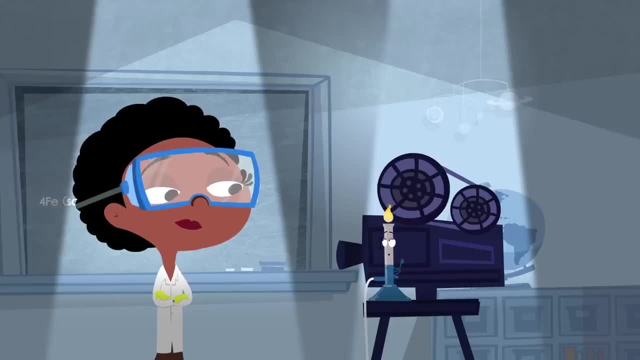 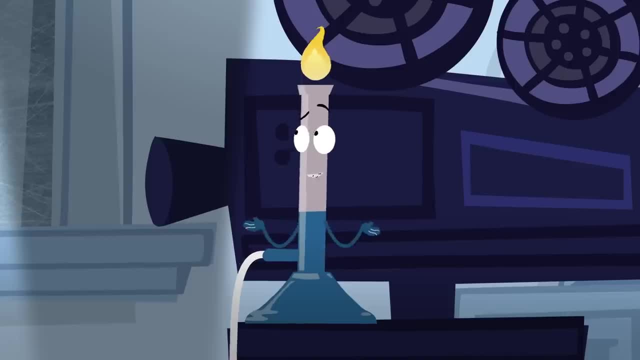 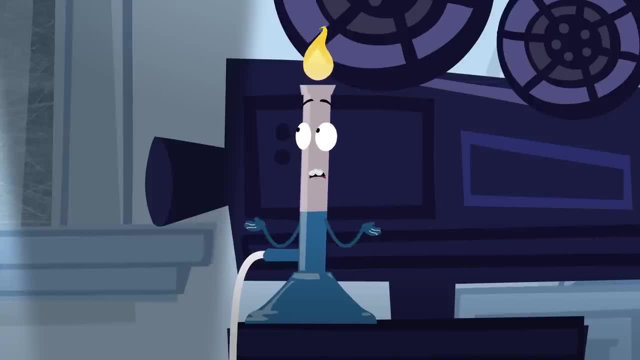 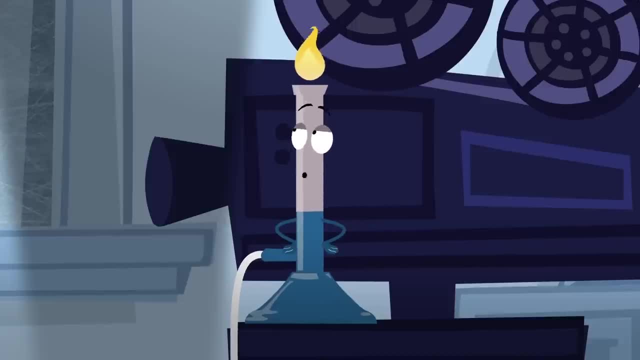 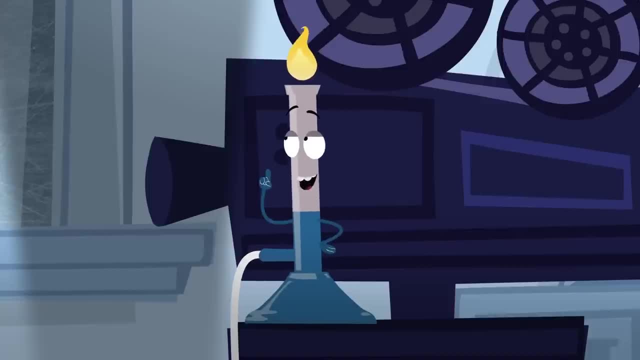 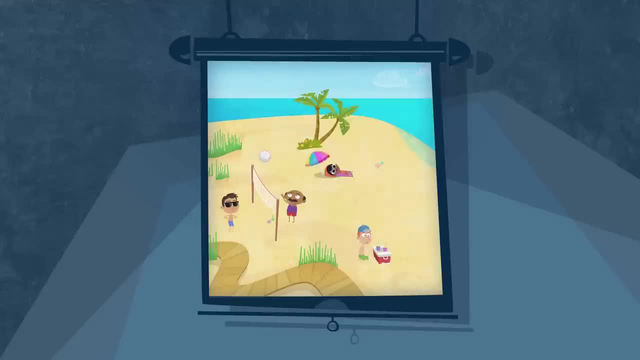 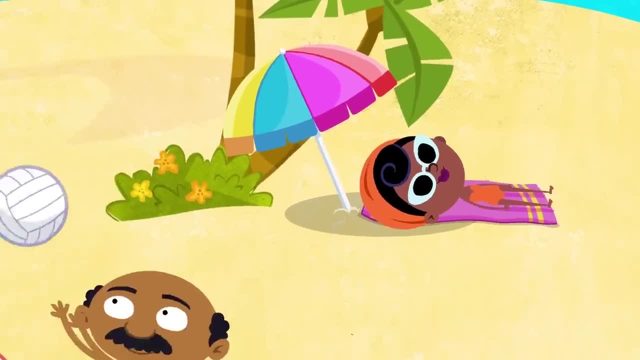 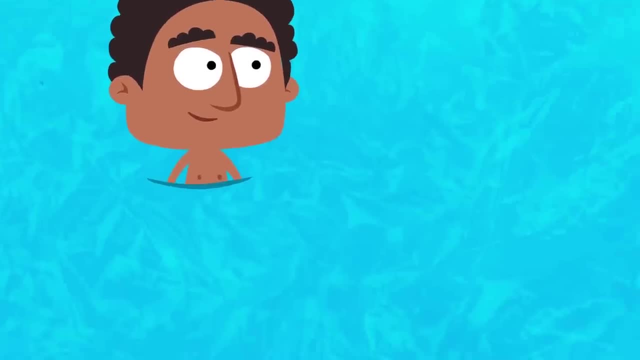 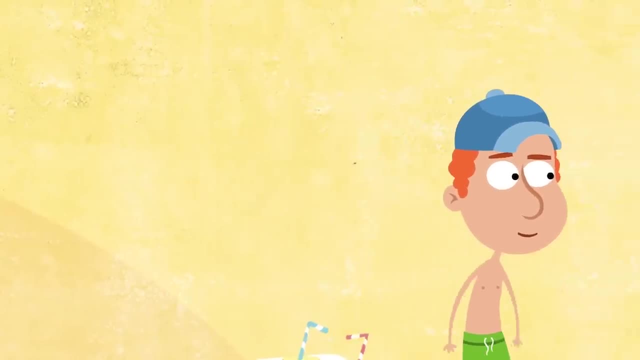 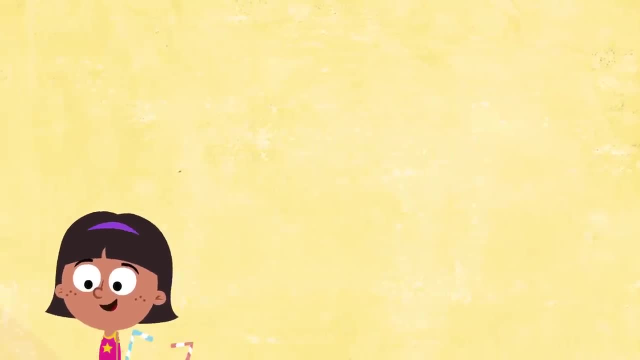 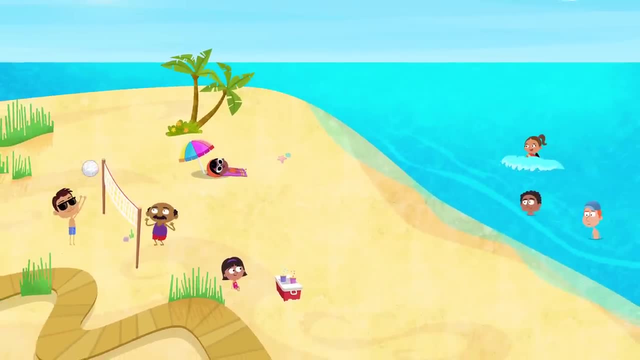 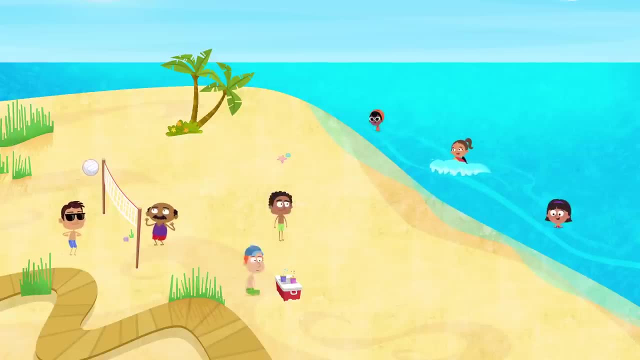 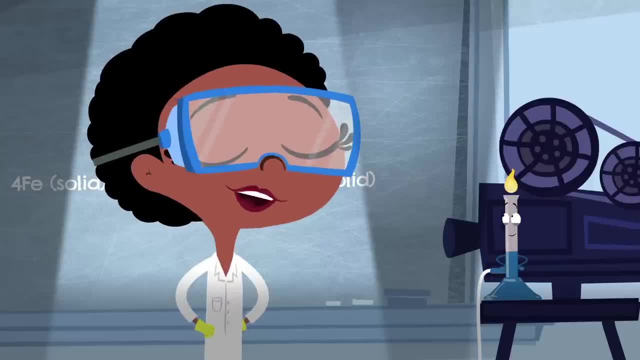 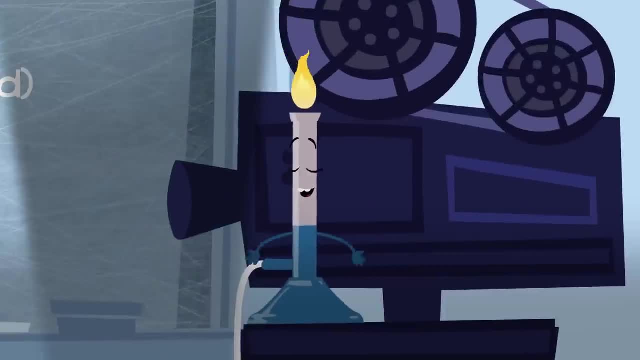 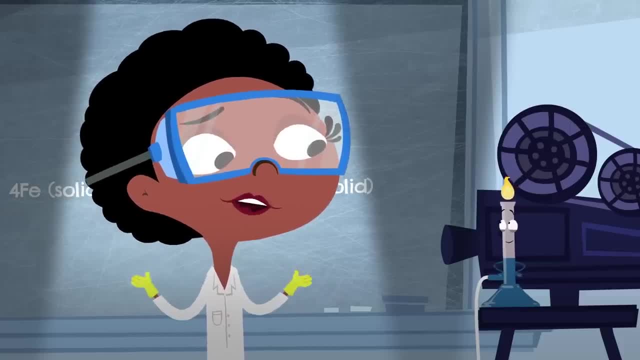 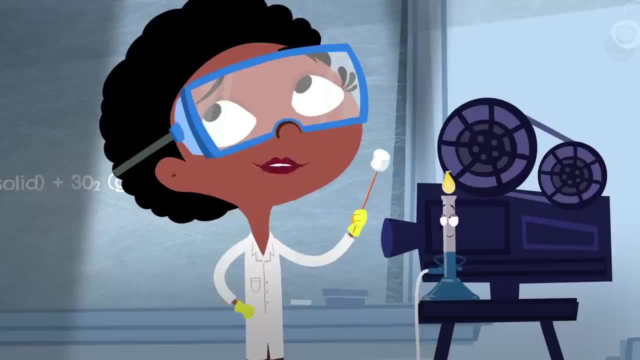 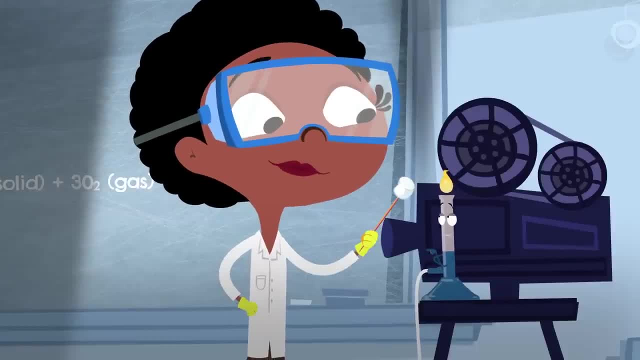 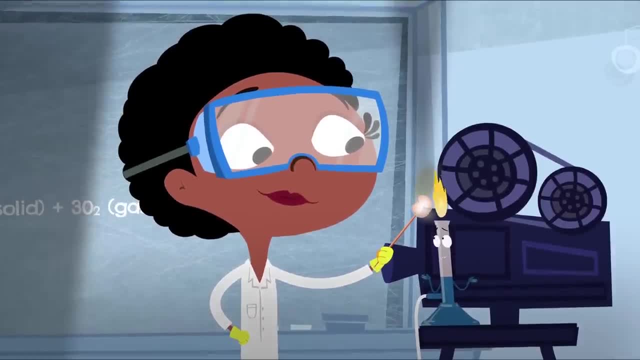 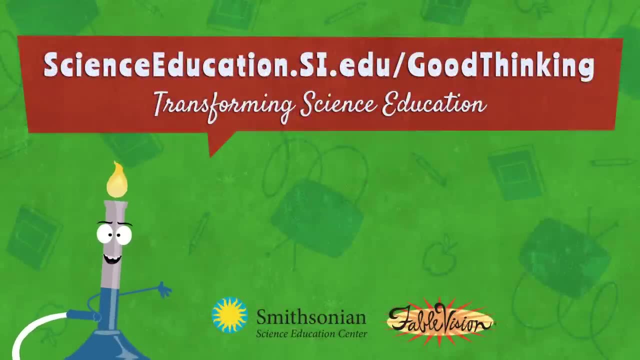 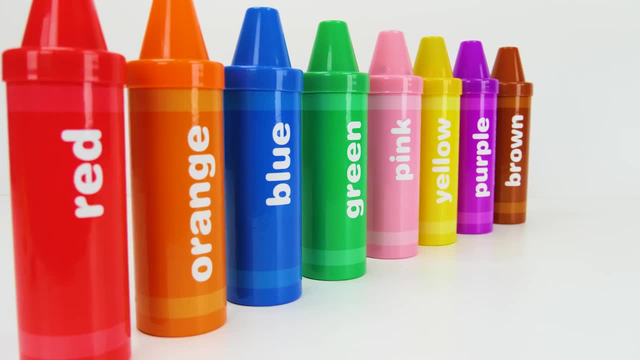 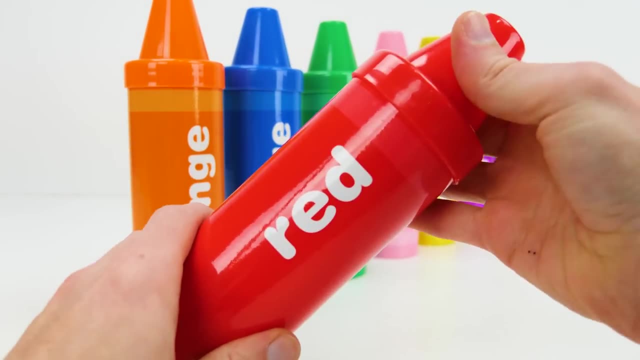 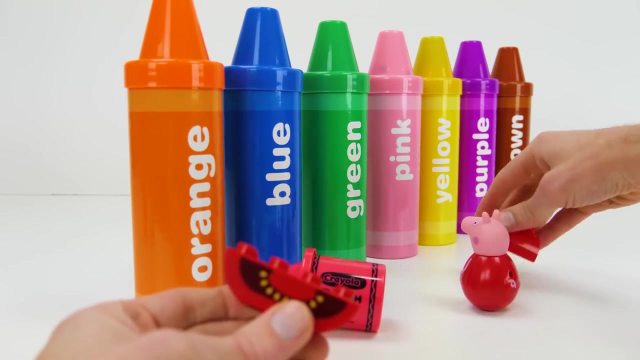 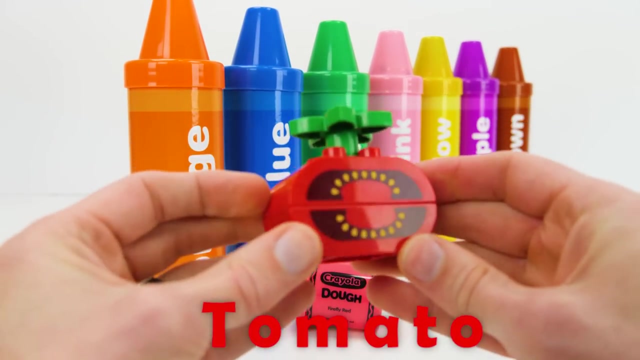 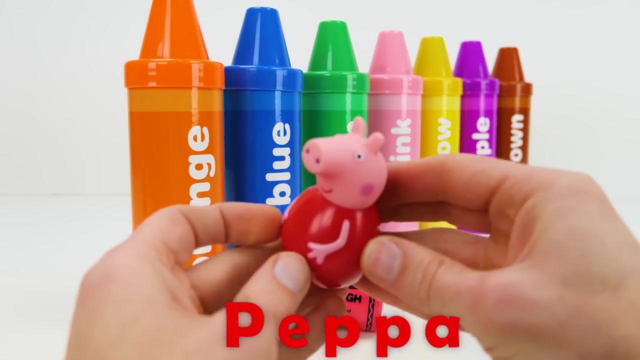 Let's see what colorful surprises are in these crayons. Our first color is red. Let's open it up and see what's inside. Wow, look at that Tomato. The tomato is tasty. Peppa Peppa can spin.